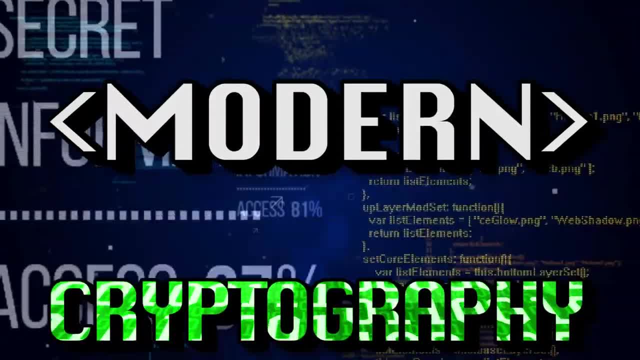 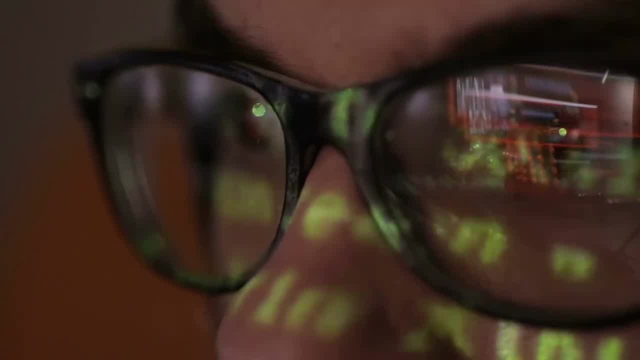 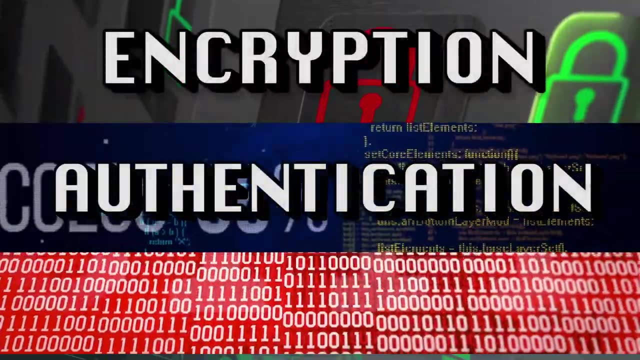 some degree, but it's also a root methodology to modern coding. Let's try to understand some basic principles of cryptology to gain a greater understanding of this old but new technological workflow. There are three key principles of cryptography: Encryption, authentication and integrity. Encryption is the process of converting data into an unreadable form in 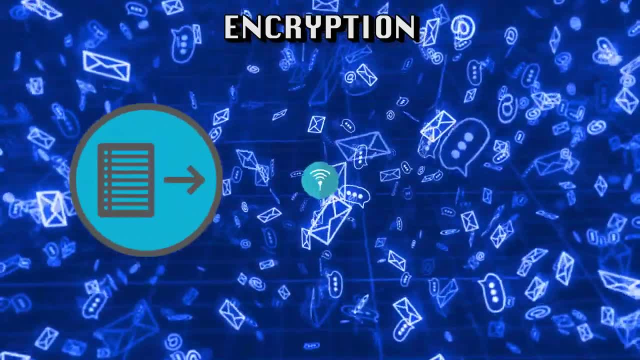 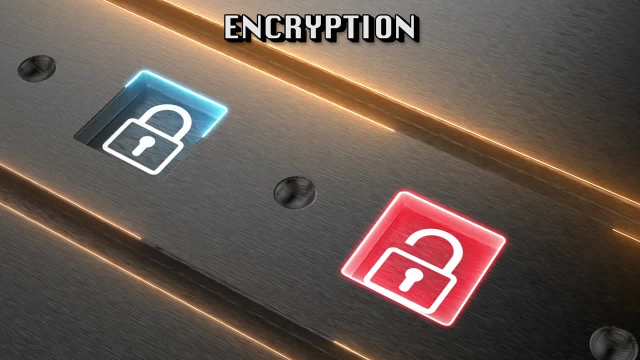 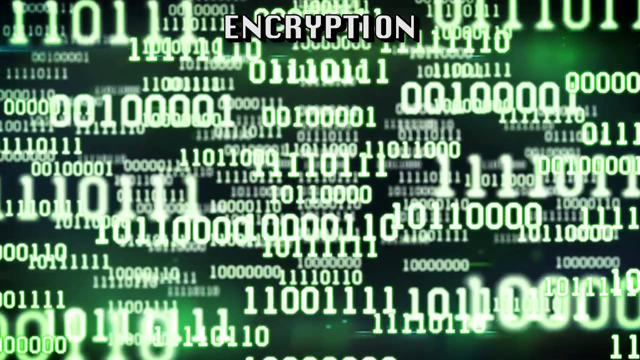 order to protect its privacy during data transfer, reception and storage. Encrypted data has to be decrypted, a process called decryption. Encryption and decryption require a key to be used In the process so that, while the data may seem scrambled, it can still be read and understood by. 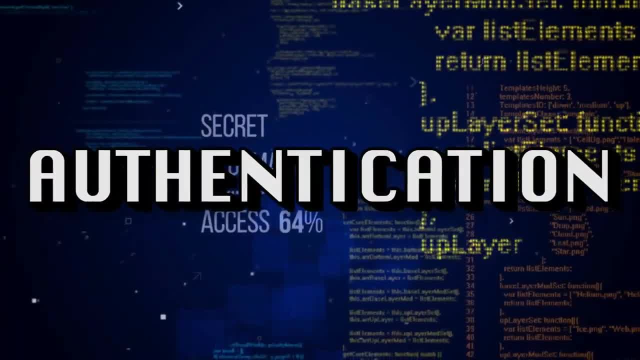 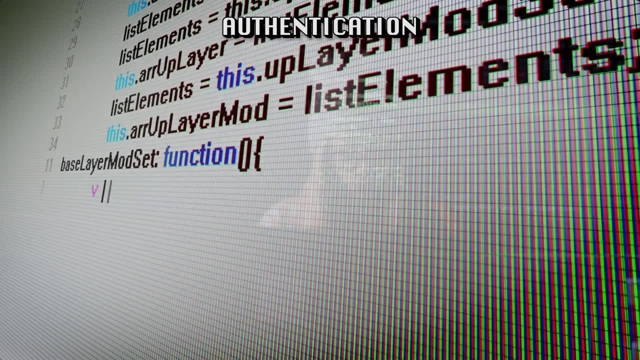 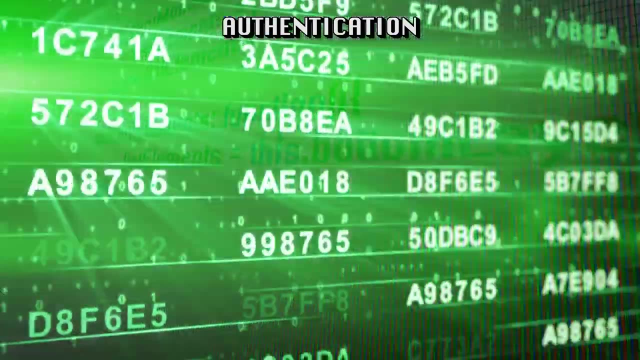 the desired recipients. Authentication is the process of ensuring that the sender claimed in a string of data is in fact the actual sender. This works by the sending computer or device performing some action that the receiver knows only the correct sender can do When the receiver 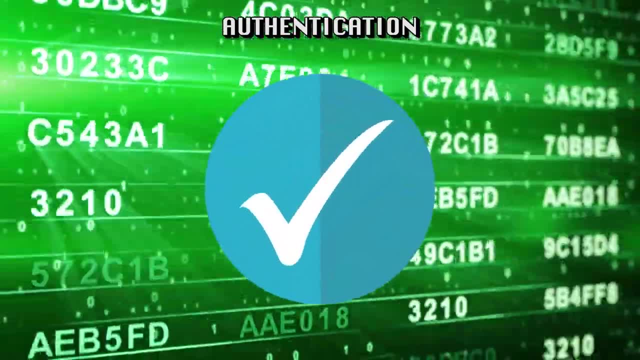 sees that action, it authenticates the message. The actual process is much more complex, but this explanation summarizes the work. Encryption and decryption require a key to be used in order to control the sender's text and display it in the right way so that the receiver can hear it. 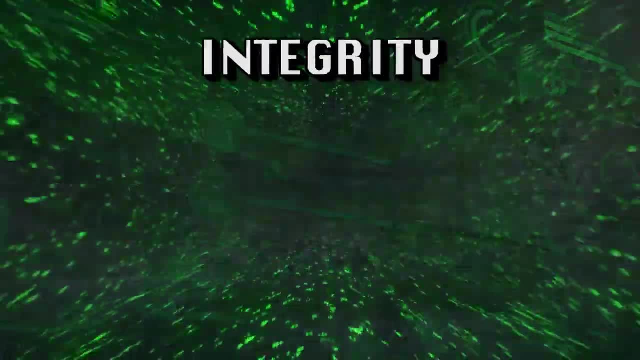 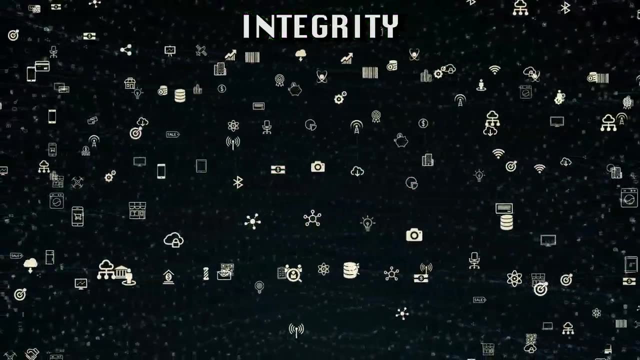 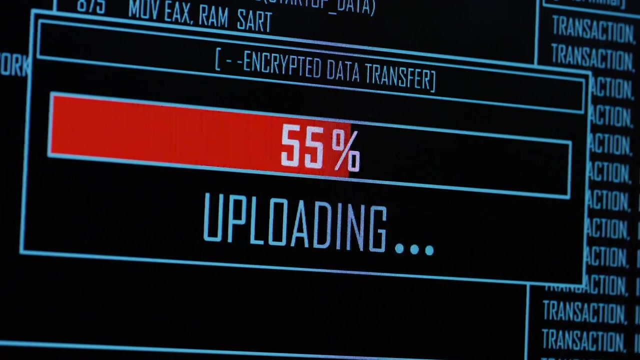 Finally, integrity. Proper cryptography also ensures message integrity, which means that the messages are communicated accurately and are not intercepted or altered on the communication path. Usually, this is done by hashing the data which cryptographically maps out its path. Taking these principles into actuality requires a wealth of technical skill, using one of three main techniques. 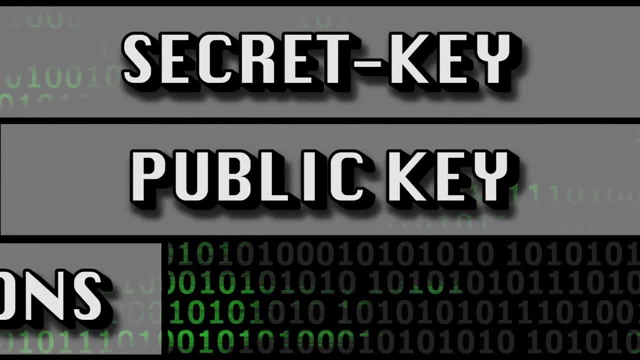 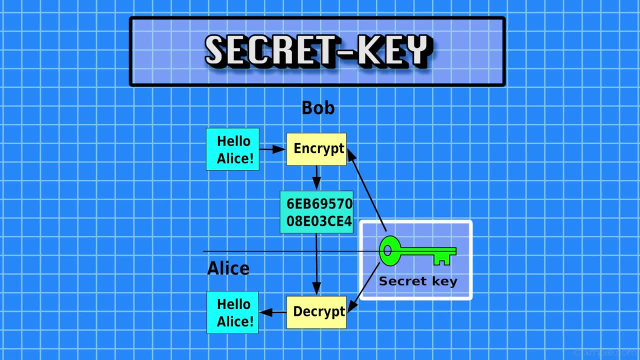 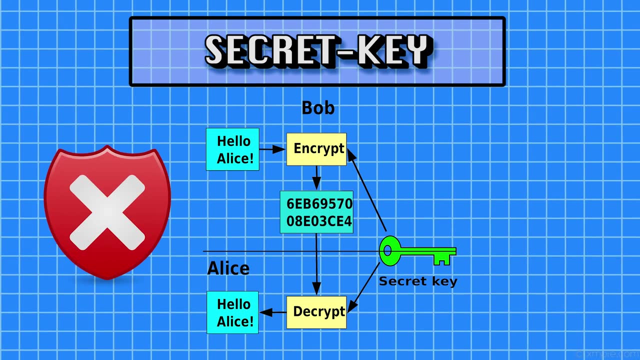 Secret Key Cryptography, Public Key Cryptography and Hash Functions. Secret Key Cryptography for cooperation with the network. Secret Key Cryptography requires a wealth. cryptography uses one key across both the sending encryption and receiver's decryption. it's the simplest way of encrypting data, but it's relatively low on security overall and distributing the 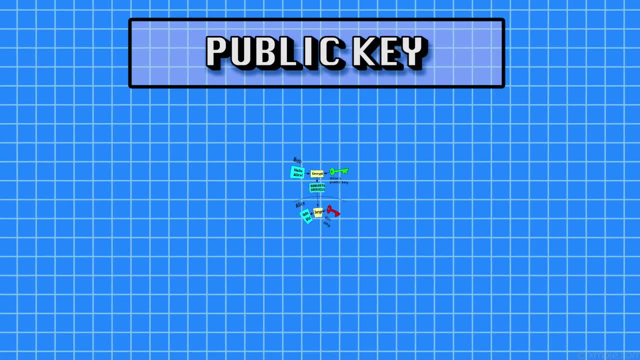 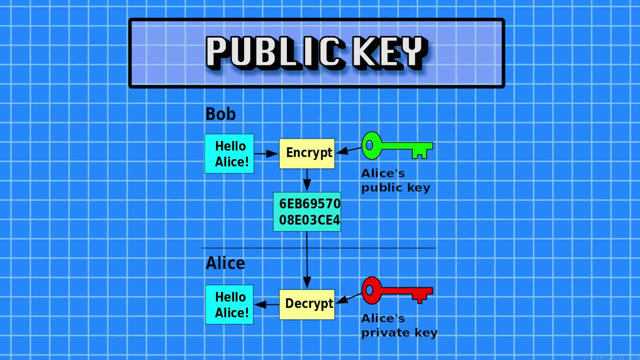 single key can often be easier said than done. public key cryptography allows for the use of two keys which are different for the sender and receiver. both the sending party and the receiving party has a private and public key. the private key should be kept secret to the individual device.